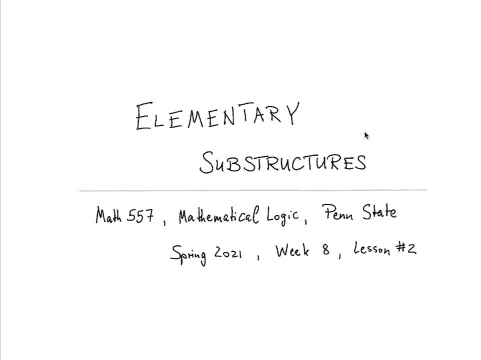 In the previous lesson we studied elementary equivalence, which meant that two structures satisfy the same sentences. In this lecture we're going to look at elementary substructures, which is the third, next to elementary equivalence and isomorphism, the third major relation between structures that is studied in model theory. 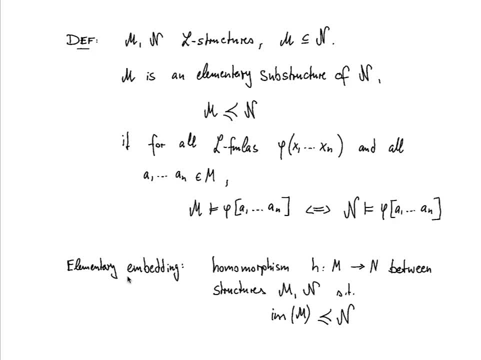 We start with a definition right away. So let's assume we have two structures over the same language, m and n, and we also assume that m is a substructure of n, Then m is called an elementary substructure of n, If for all L-formulas, phi, with three variables among about. 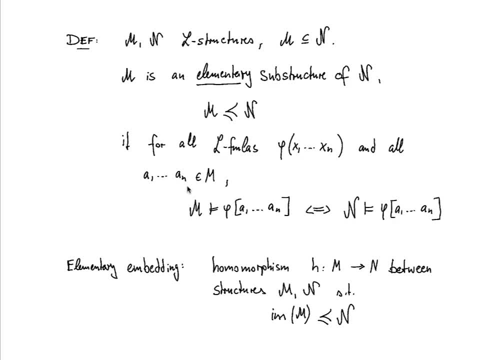 x1 up to xn and all n elements of x1 up to xn are true under the assignment a1 up to an from m. that formula phi is true in m under the assignment a1 up to an, if, and only if, it's true in n under the same assignment. 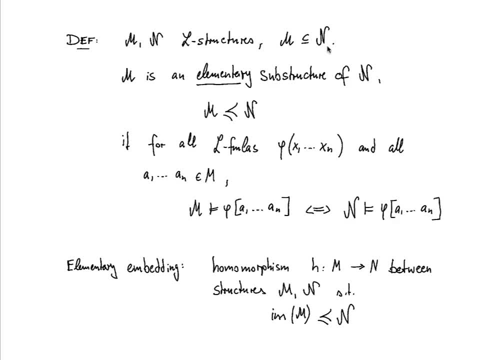 Keep in mind that m is a substructure of n, so this makes sense to write this here. So the difference between elementary equivalence and elementary substructure is, of course, first of all we need to assume here for this definition to make sense that m is already a substructure of n, But then the property here is definitely stronger. 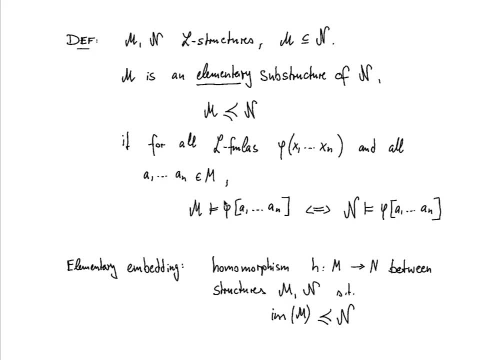 than being just an elementary equivalence, because we now can also look at formulas that are not sentences but just formulas, and also plug in values from the smallest structure And look at the satisfaction relation with respect to those formulas between n and n. We can extend this, of course, away from substructures to consider. 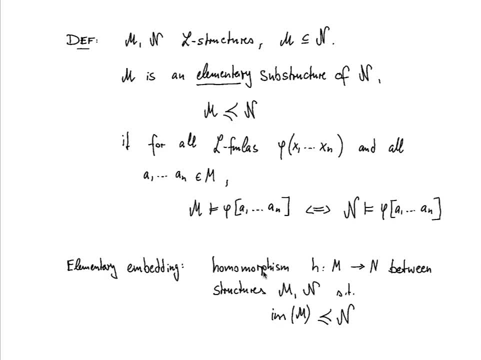 the notion of an elementary embedding. That holds if there is a homomorphism between the two structures and so that the image of that homomorphism is an elementary substructure. So if we can choose a homomorphism for structures, recall that means we can. 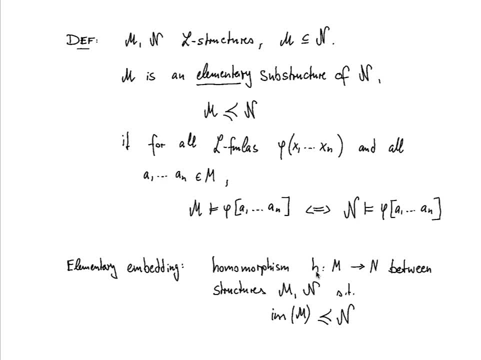 define a mapping that preserves essentially all functions, constants and relations between m and the image And, if we can choose a homomorphism, so that we can actually embed m into the bigger structure, so that this relationship between m and the image is actually a substructure of n. 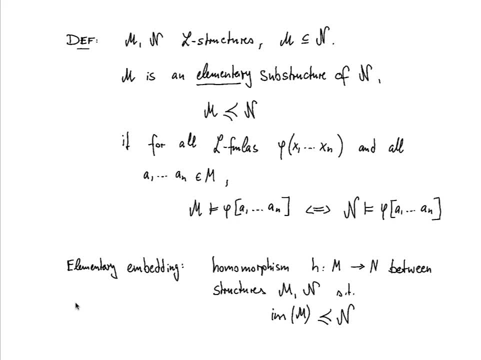 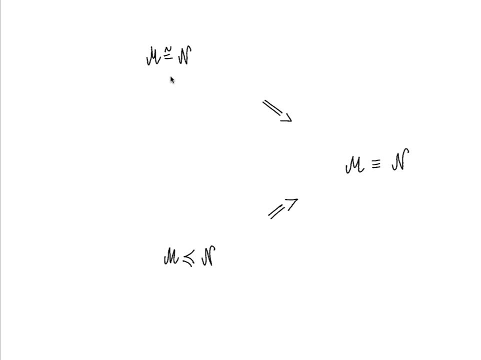 So we can see that m is an elementary embedding and that the elementary substructure relation holds the elementary substructure relation holds, Then we call that an elementary embedding. So we now have two notions that both imply elementary equivalence. We've seen that. 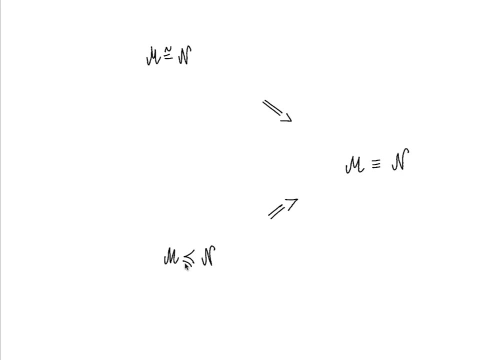 isomorphism always implies elementary equivalence, but not vice versa. Similarly, as can be easily seen from the definition, being an elementary substructure also implies being an elementary equivalent to the bigger structure. So if we can define a homomorphism that we can actually embed m into the bigger structure. 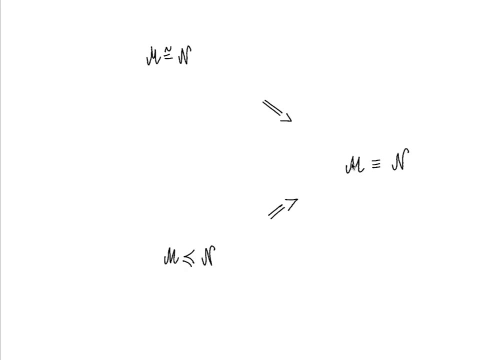 And, if we can define it, that we can actually embed m into the smaller structure, because here we actually look at all kinds of formulas, Whereas here we would only have to look at sentences. The notion of isomorphism and elementary substructure in turn are not comparable. 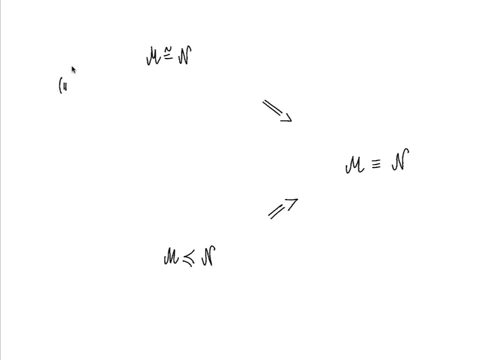 So we can have one without the other, one holding or implying. So for example, look at the two structures: is the natural numbers. we take out 0 and also look at the less than relation. So these two structures are obviously isomorphic if we map n to n plus 1. but 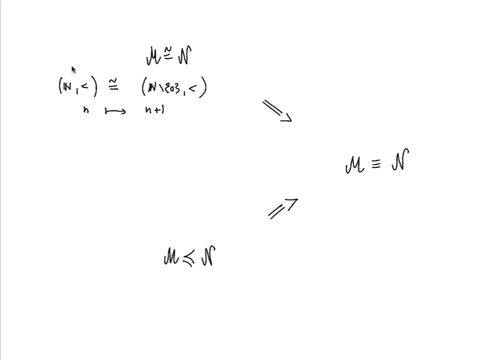 now we could look at the formula with one free variable, phi of y being not, exists x, x less than y, and then if we put y equals 1, then we see that this structure here n without 0 less than that satisfies phi of 1, but the other 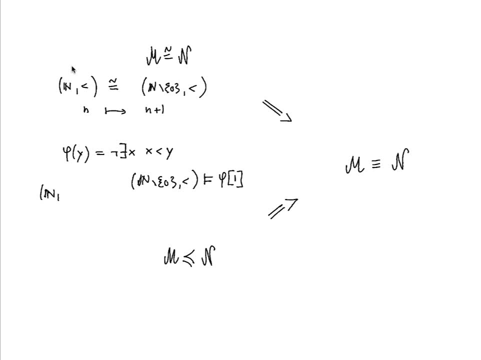 structure n less than does not satisfy this phi of 1 here. On the other hand, we will later see that the linear order Q is an elementary substructure of the linear order of R, and of course these cannot be isomorphic simply for cardinality reasons. 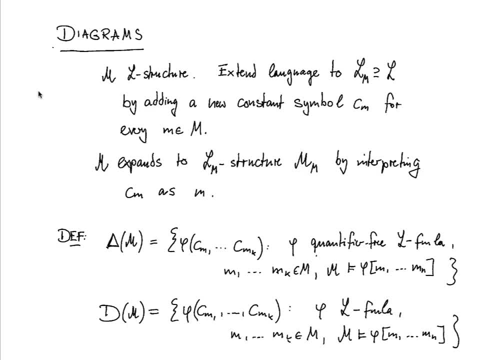 So we have seen that, for being an elementary substructure, a crucial property was that we could actually now address in our formulas specific elements of a structure. It is possible to do something similar or analogous on the syntactical side by introducing additional constants to the language. 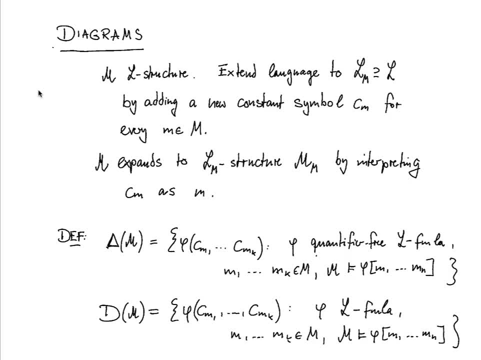 that represent the elements of a specific structure And um that is called the diagram method. So suppose we have an L structure and we extend the language from L to LM by adding a new constant symbol. so a new constant symbol, CM, for every m in M. 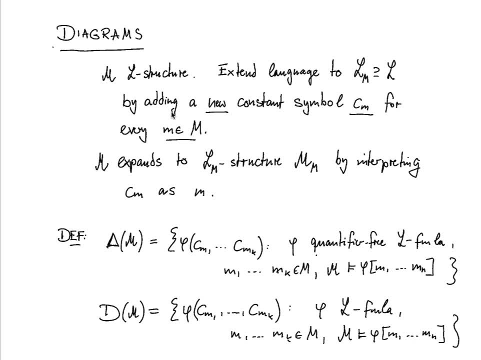 Right. So we just take for every element in our structure, we just add some constant symbol to the language right, And now we're able to address every element of this number right in this structure, and that's all we have here. I hope you like this video and I hope you. 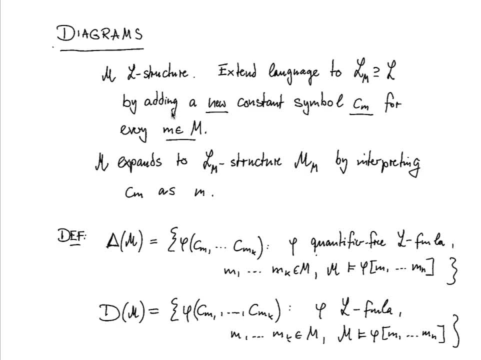 element of a structure in a formula directly, by just interpreting the constant symbol c m as m, And this way we clearly can expand a structure m to an lm structure m sub m, again by interpreting c m as m, And then we can form two sets of formulas. The one here is delta m, That's the set of 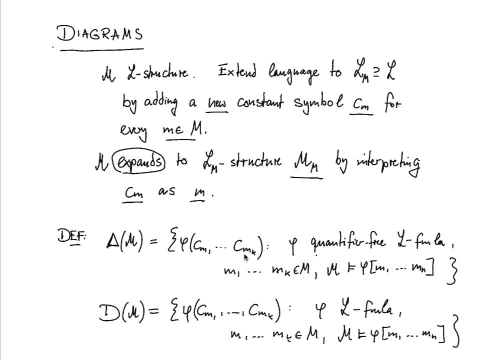 all formulas- phi, c, m1 up to c, mk, where phi is quantifier-free. So that's important here. That is a quantifier-free l formula And m1 up to mk are elements of m, such that if I assign m1 up to mn to these positions here, 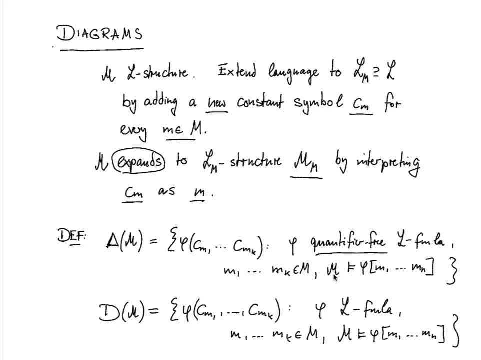 then this formula, phi, holds in m. So this is also called because we are restricting ourselves to quantifier-free formulas. this is called the simple diagram, Whereas the next set of formulas doesn't have such a restriction. So if we look at any l formula here and form the same set of formulas, only we drop the restriction. 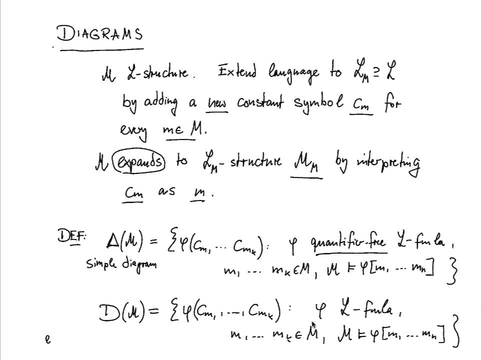 on quantifier-free, then we get what is called the elementary or complete diagram of M. You can think of a diagram as recording all facts about a structure that you can write down using the symbols in your language, right? So it's a little bit like a generalization of a group multiplication table. 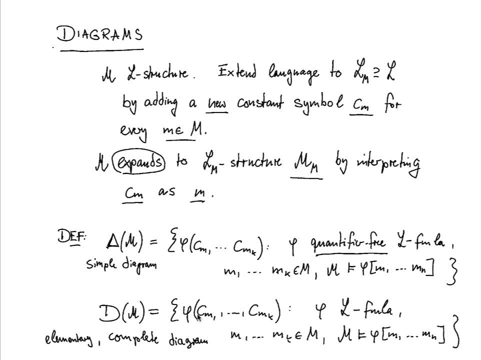 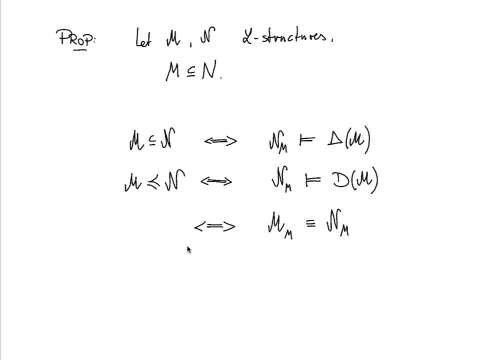 where you also record all the different relations between the elements with respect to the group operation. The nice thing about these diagrams and the extended language is that you can now capture model-theoretic notions between structures using the satisfaction relation and the model relation for. 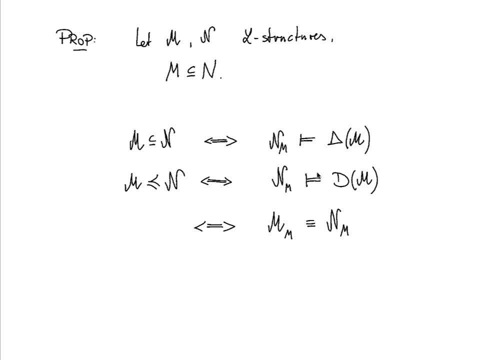 structures and sets of sentences and formulas In particular. so let M and N be L-structures and let's assume that M is a subset of M, So the universe of M is contained in the universe of N. Then M is a substructure of N. 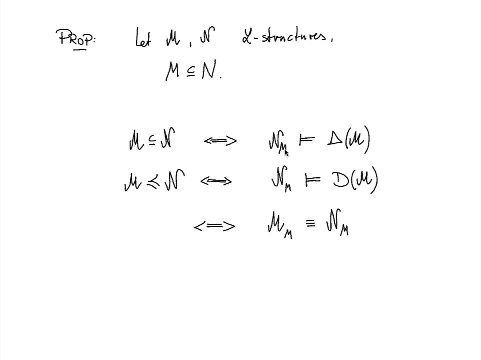 if, and only if, N when interpreted as the expanded structure. so we expand the language, add a constant element for every element of M and then interpret that constant element back as the corresponding element of M if that structure satisfies the simple diagram of M. 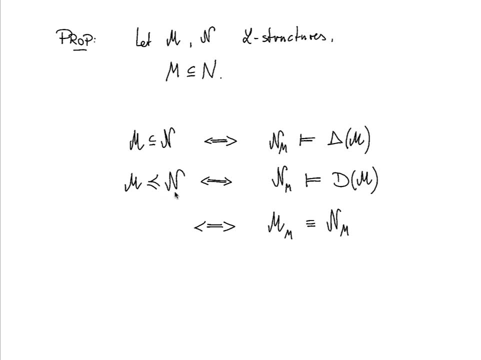 Furthermore, M is an elementary substructure of N if, and only if, this expanded structure, N sub M, satisfies the elementary diagram of M And this then becomes equivalent to the expanded structure being elementary equivalent now. So, because we can now actually address single elements of the structures in our language, 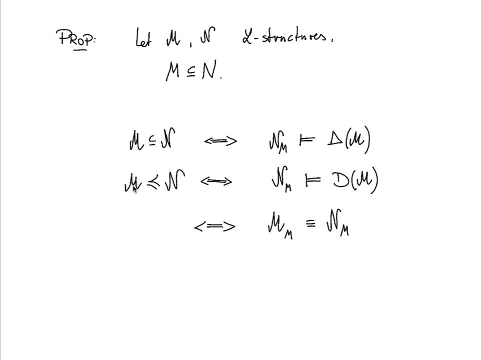 which we need to express, element being an elementary substructure. this now, we can characterize this via elementary equivalence of those expanded structures. And this is just an example that I can give you Regarding the proof of these facts. the proofs of these facts are not very hard. 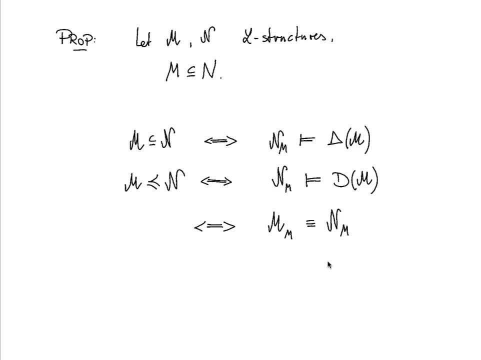 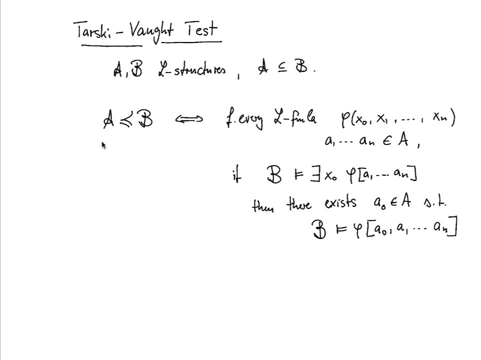 pretty much straight forward from the definitions, But, as always, I recommend you sit down and walk through the few steps yourself. The definition of being an elementary substructure may seem a little daunting at first because in order to check it, we need to verify the truth behavior for every formula. 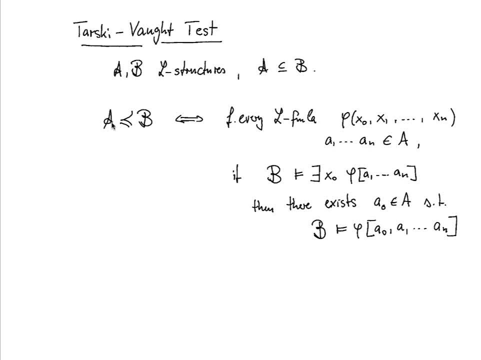 and for every tuple from the smaller structure. However, this can be greatly reduced to checking only a certain kind of formula and for a certain kind of witness, And this is called the Tarski-Vaught test or criterion. And that test says that A is an elementary substructure of B. 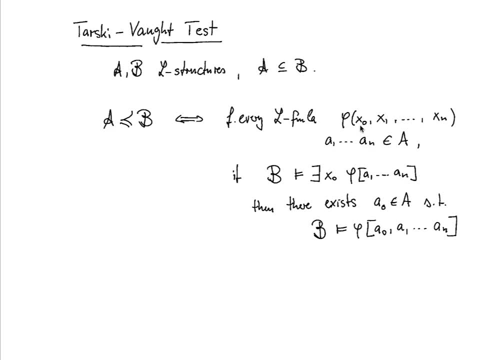 if, and only if, for every formula phi in free variables x0 up to xn and n-tuple A1 up to An from the smaller structure. If the bigger structure satisfies an existential statement with x0, phi, now with assignment A1 to An. 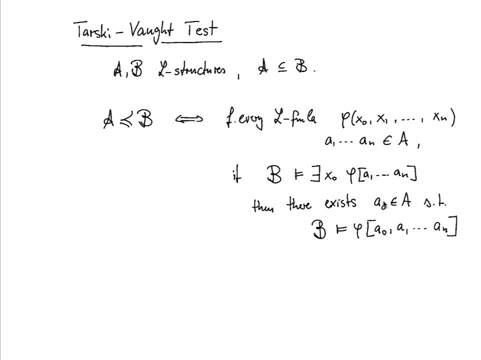 to the remaining variables. then we can find a witness for that existential statement already in the smaller structure A. So there exists an A0 in A, such that it is an elementary substructure of B, which that B satisfies that statement with assignment A0 up to An. 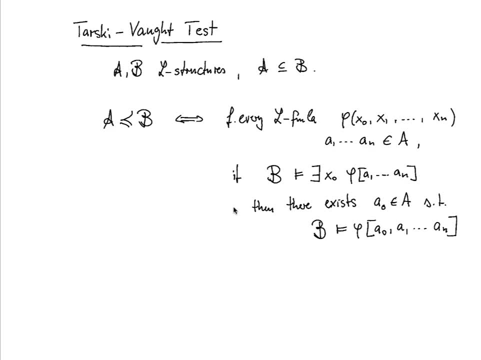 So, when checking for being an elementary substructure, we can actually restrict ourselves to just checking this property, this witness, property for existential sentences or formulas And the proof. as usual, I encourage you to try to find it. So let's go ahead and check this. 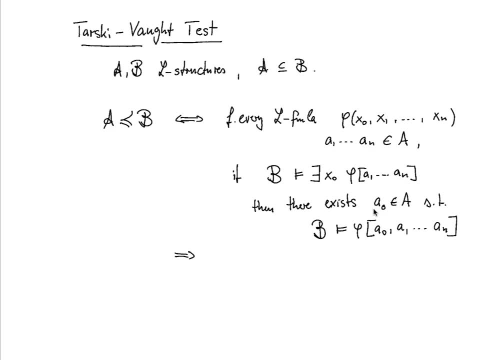 Let's go ahead and check this. Let's go ahead and check this. Let's try to work this out yourself. So this direction is more or less clear. It follows almost immediately from the definition of an elementary substructure, whereas this direction proceeds by induction. 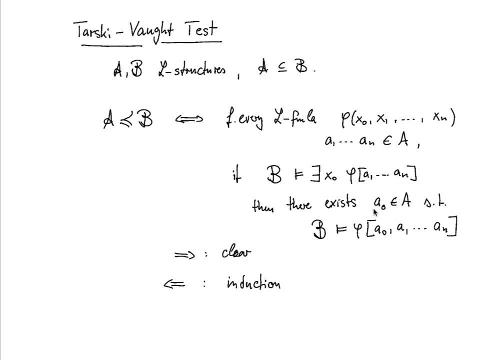 on the height of the formula phi And most cases, again, are not difficult, Only the case where we do an induction on the height of the formula phi and the induction step going from a formula to an existentially quantified formula. 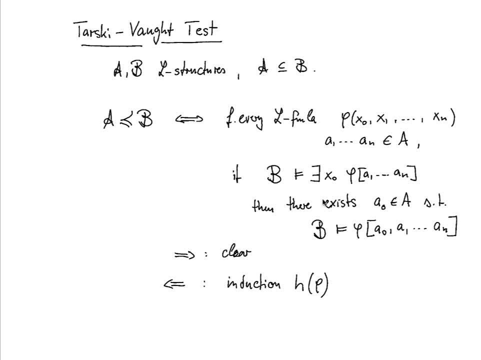 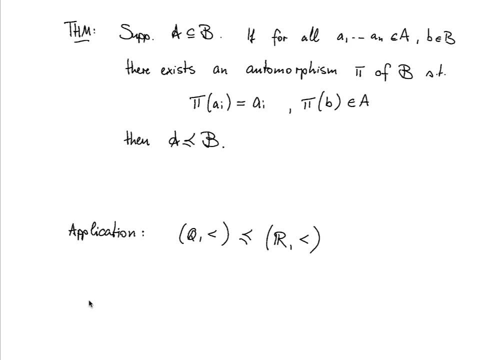 that is where we need to do some work, And this is precisely the case where the criterion helps us to make that induction step. The Tarski-Vaugh test yields also the following criterion for being an elementary substructure, Namely if we have A given as a substructure of B. 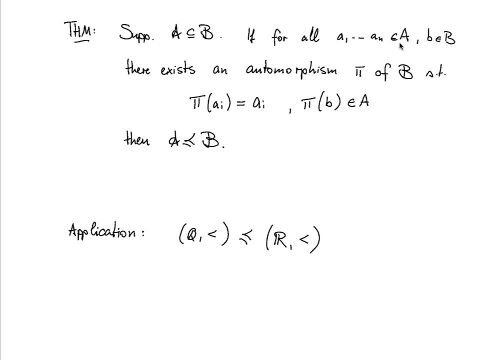 if for all A1 up to An in A and B in B, we can find an automorphism pi of B such that this automorphism leaves the Ai's fixed and moves pi in B into A, then we have an elementary substructure. 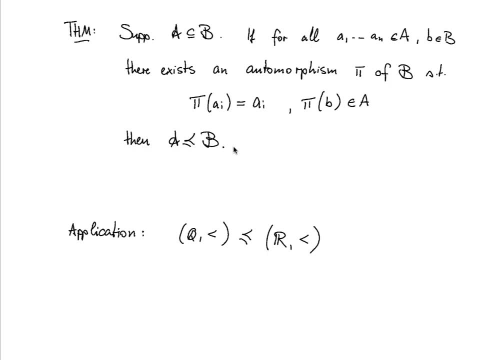 So again, if we do have a structure B here, and inside this sits A, and we can find an automorphism given a set of a finite tuple in A- let's say in this case A1,, A2,, A3, and an element B in B. 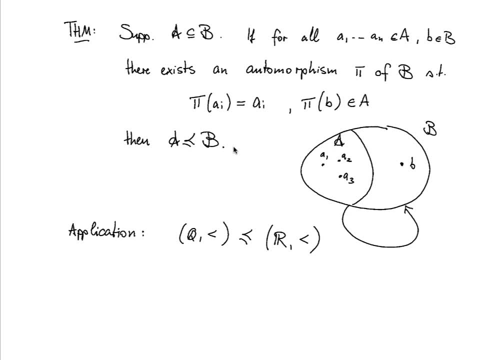 we can find an automorphism pi of the structure B that leaves the Ai's fixed and moves B into B. So we have an elementary substructure of B into A And one application of this, and of course you should see that you can verify this theorem.